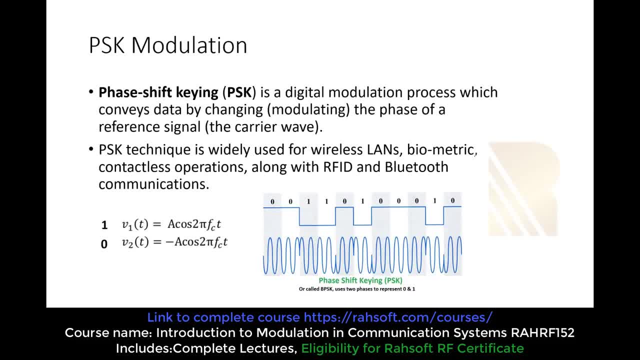 PM, the phase modulation, So a phase shift keying, or PSK, is a digital modulation process which conveys data by changing or modulating the phase of the reference signal. What is the reference signal? Of course, it's our carrier. So we have a carrier which has, which is a five. 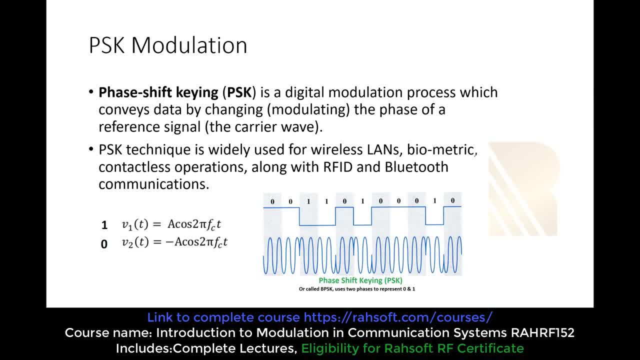 frequency signal and we have a binary data. We are trying to send this data by changing the phase of our carrier. So in this part we are going to talk about the two level PSK signal. So, uh, we say the when the PSK signal is a two level- We talked about this- we say the beat rate is equal. 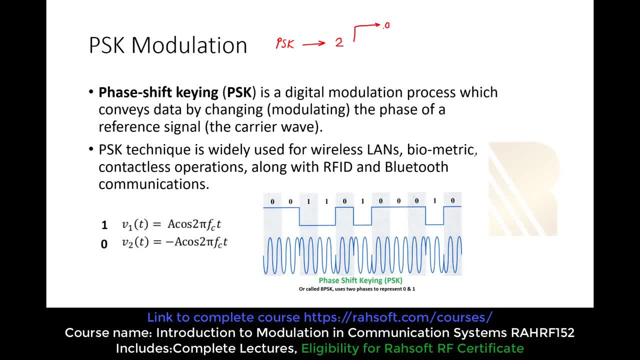 to baud rate and we have two levels: the- the zero means the zero and the one data from the binary side. so we are going to call this bpsk- bpsk. so this is actually the psk and bpsk. they're they're same thing. they don't have any difference. so we can see in this picture what is going on. 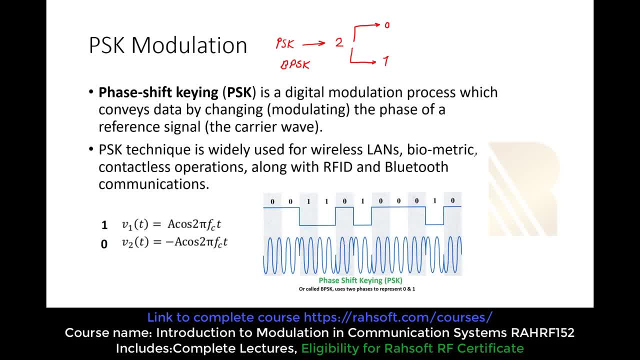 here. uh, how can we modulate the um, the data here? so we're going to say: imagine that we have a binary data of for this one, actually for bpsk, we have a binary data of 1 and 0.. so it's very simple. 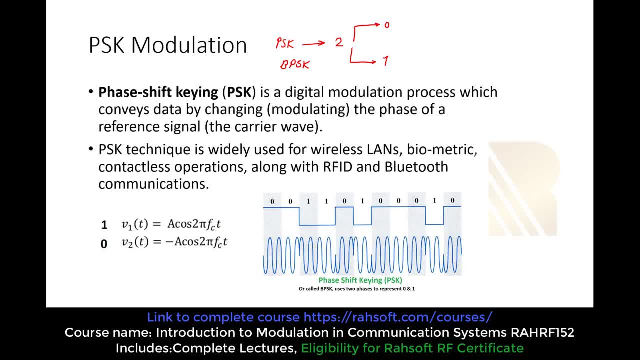 when the data is 0, we are going to send minus a cosine 2 pfct, and when the data is 1, we are going to send a cosine 2 pfct. so you can also see in this picture- it doesn't matter this, this also. 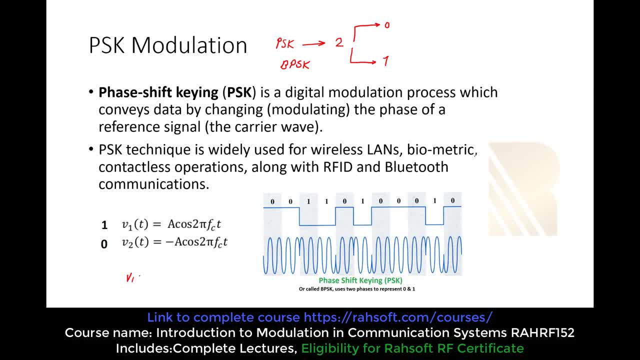 can be a sine wave. so example, for example: then v1, v1 can be, let's say, a sine omega ct, or um for the. this is for one, and when we are sending zero, the v2 can be- uh, the minus- a sine omega ct. so it doesn't matter if you have a cosine or sine here. so, as you see in this picture, 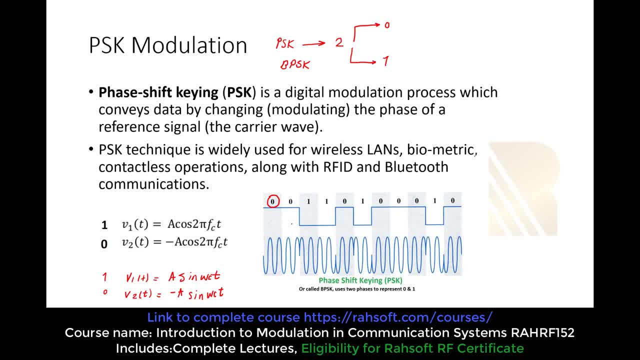 when we have a zero as our data, as a binary data. here this is a binary sequence. again, here we are going to send the minus a sine omega ct, as you see here. so again we are sending the minus and at this part we are, we have one. so the phase is changing, as you see at this. 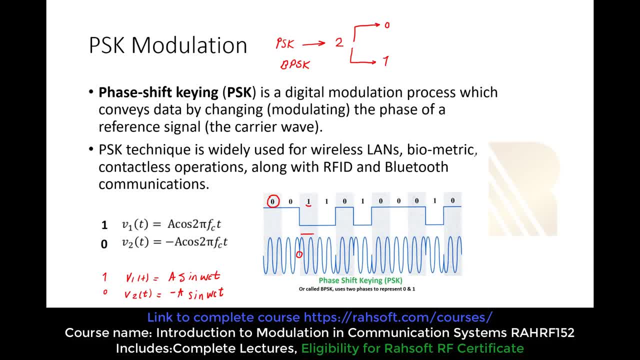 point. this is a phase shift. and now this: as you see, this signal here, the wave here is the sine itself. so this is minus sine wave. minus sine wave, um or minus a, it doesn't matter. i'm assuming the amplitude is one. so this is sine sine again, um. at this point, as you see, is changing the. 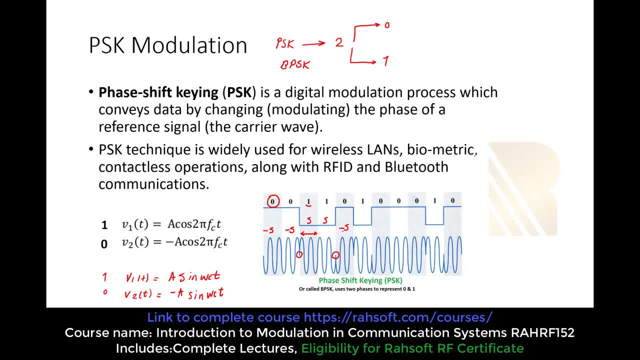 so we are, uh, sending the minus sign for zero, but then. but then now the question is: uh, you'll say, okay, if this is a phase modulation, then why we have a different amplitude. so, as you see, in this two waves the frequency is constant, but the the amplitude is changing. but the answer 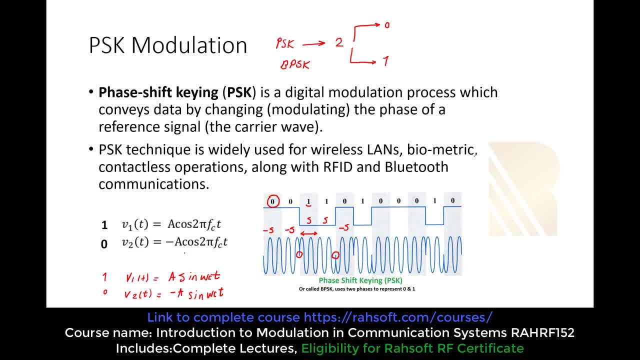 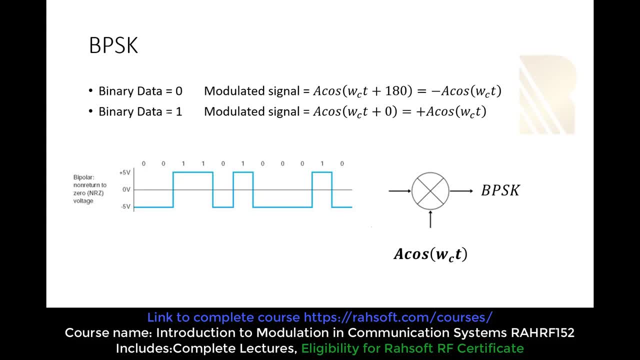 is: uh, yeah, it's kind of tricky. it's not like that. the amplitude is not changing, the phase is changing and we are going to explain about this. so what is going on? when we send the binary data zero, we send the modulated data signal as a cosine: omega ct plus 180 degree phase shift, or we can say it's plus. 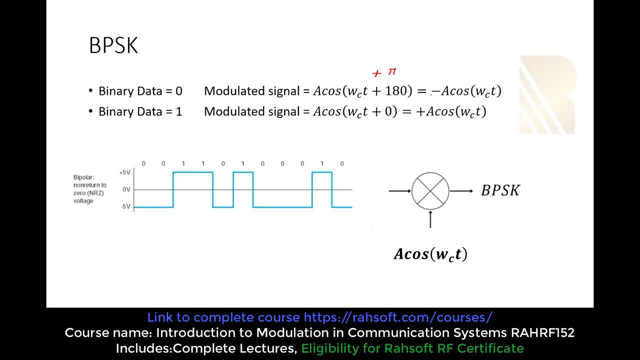 pi here. so then this: we can write this as minus a cosine, omega ct. so the amplitude is not changing, the phase changes. we send it with the 180 degrees of phase shift. that's why this is going to be negative because of that, this sign. but uh, this is for bpsk, so we have two levels. 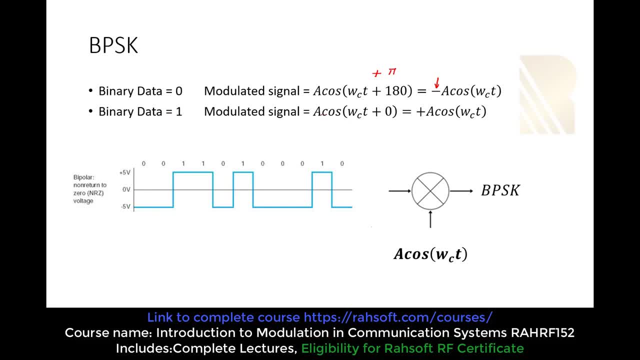 in the second level, when the data is one, the modulated signal is going to be a cosine omega ct plus zero, the zero phase. so then it's going to be the same. so that's why, if you're writing minus a cosine omega ct plus a cosine omega ct, but the real uh scenario is we are going to have a 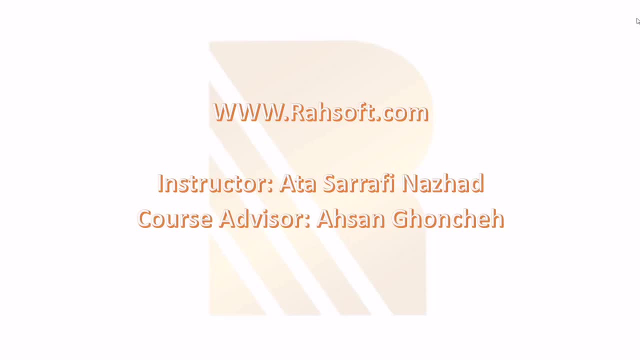 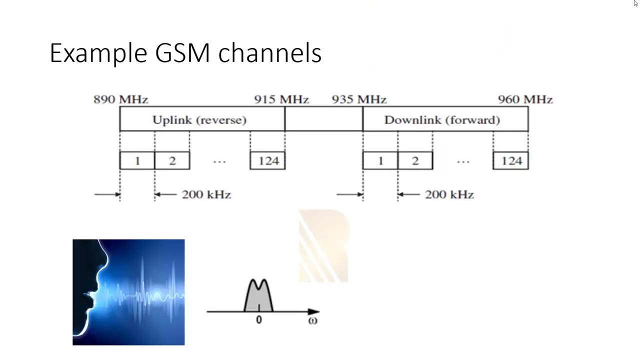 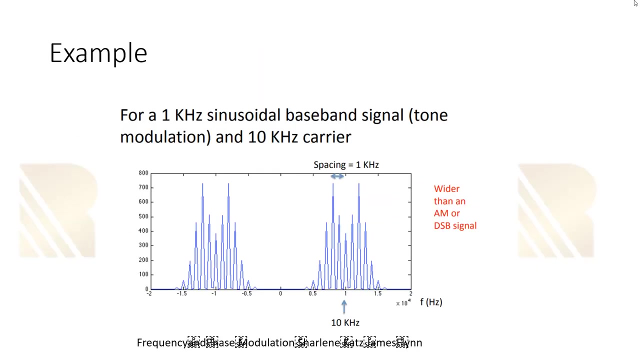 phase difference. thank you for watching our video. please don't forget to subscribe. you can learn about this topic and more using our website. the complete course on this topic is provided on our website at wwwrasoftcom. rasoft is providing a complete certificate on radio frequency.